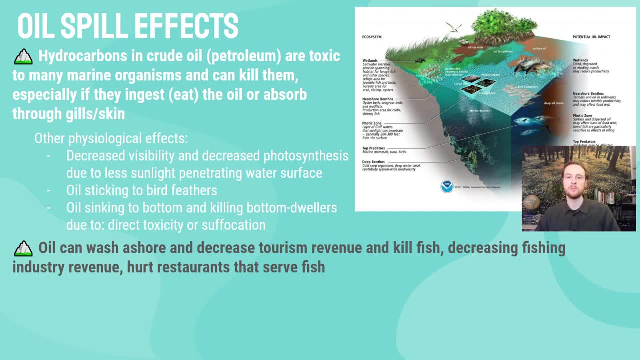 ocean. we also have some economic impacts that humans are going to suffer in these coastal communities. So when oil washes ashore, likely beaches are going to be shutting down. Tourism revenue is just going to plummet. People don't generally like to go and look at an oil spill. They can't really enjoy the 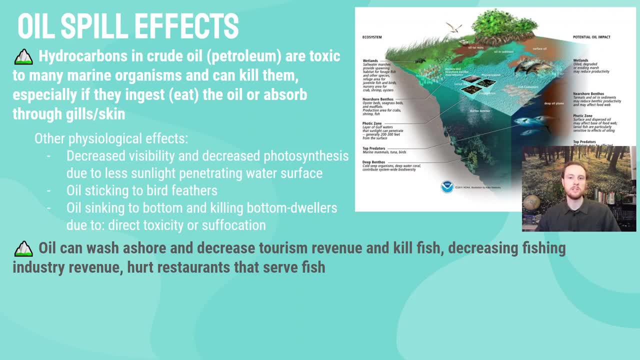 beach And then also the fishing industry, So the people whose livelihoods depend on catching fish and selling them to restaurants, but also the restaurants that depend on serving those fish to tourists. So a lot of effects that are going to occur economically for the people who are. 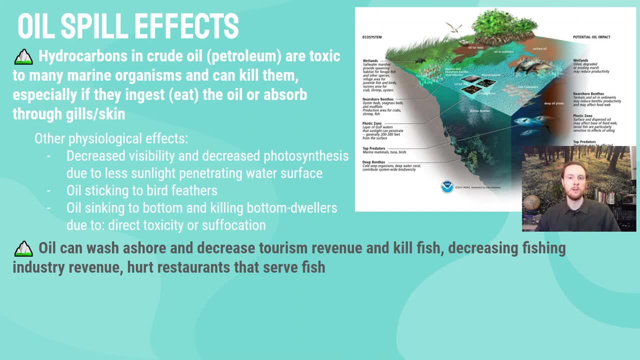 living in these coastal areas and the human communities along these coastal ecosystems as well. What we want to do now is focus on some estuary impacts. Remember that an estuary is a salt marsh or a mangrove, some sort of basically partially salt and partially freshwater ecosystem along the 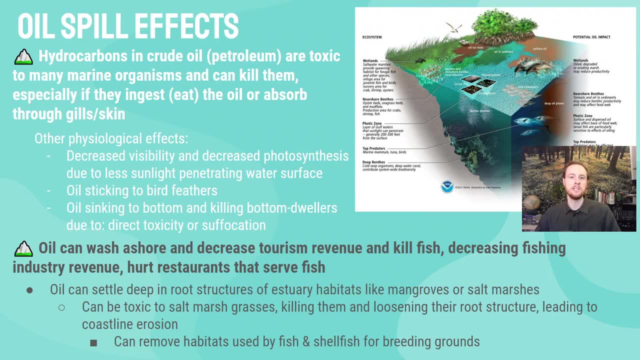 coastline of an ocean. And so what's going to happen is the oil is going to penetrate deep within the root structures of these very sensitive salt grasses and, you know, mangrove trees, and it can basically poison the plants, stunt the growth, The plants can eventually die and when they die, their root structure starts to break down and that 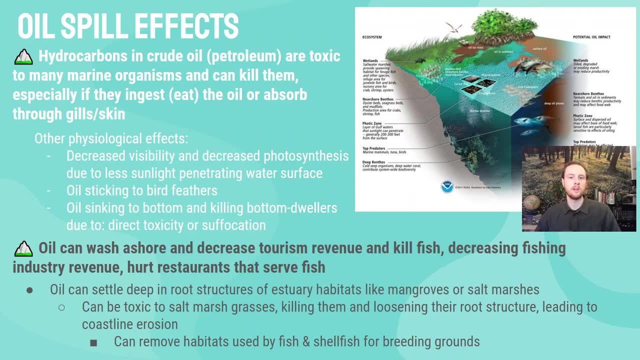 root structure is really critical for a couple reasons. One, it's oftentimes going to be a prime habitat for the breeding grounds of many fish and shellfish. So even if fish and shellfish communities aren't decimated directly by the oil being toxic, their breeding grounds may 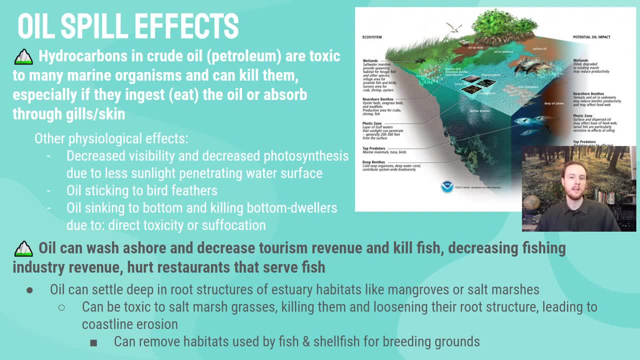 start to deteriorate. So there may be long-term effects, decades down the road, on these fishing industries that depend on these fish. Also, when these grasses and when these mangrove trees start to die if the oil penetrates their root structures too deeply. the coastline 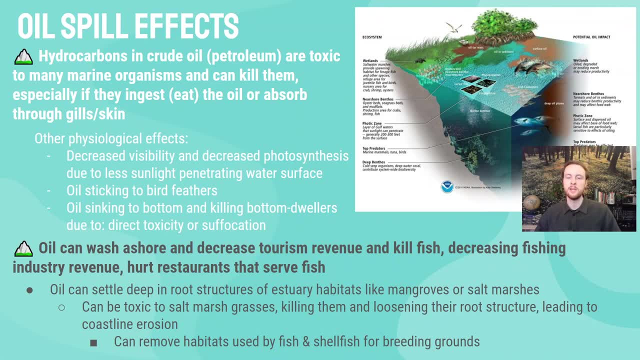 itself can start to erode, because those plants are so critical at stabilizing the coast and anchoring it with their root structures. So really, really broad reaching effects here of oil spills when it comes to the organisms themselves, human economies and also just the structure of the 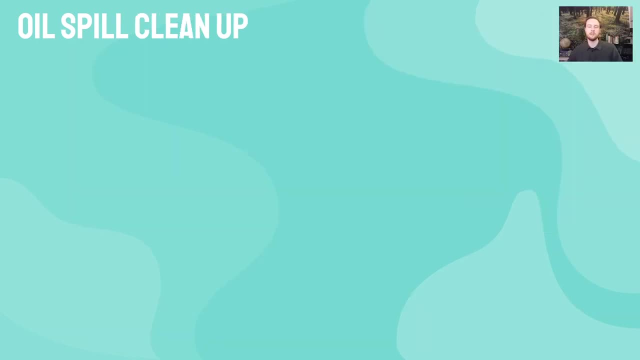 coastline itself. And finally, we'll wrap up today by talking about how oil spills can be cleaned up. So the first thing we want to note is the major ways that oil can spill into the ocean, And there are two major ways. One is a. 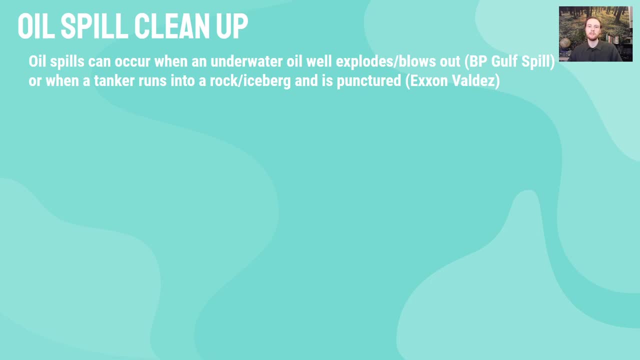 wellhead explosion or a blowout. This is what happened with the Deepwater Horizon, the BP oil spill. Basically, the well actually exploded and the oil just started leaking out into the ocean from the ocean floor. We can also have a tanker, though, which is a large ship that transports crude. 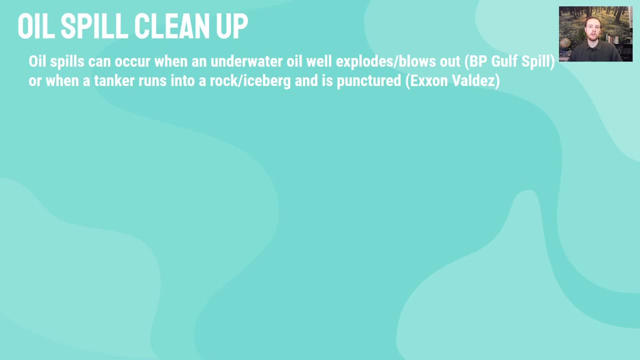 oil, usually to a refinery, and those ships can run aground. They can hit an iceberg, they can hit a rock, and this happened with the Exxon Valdez that's probably the most famous and the largest oil tanker spill. So two different ways. 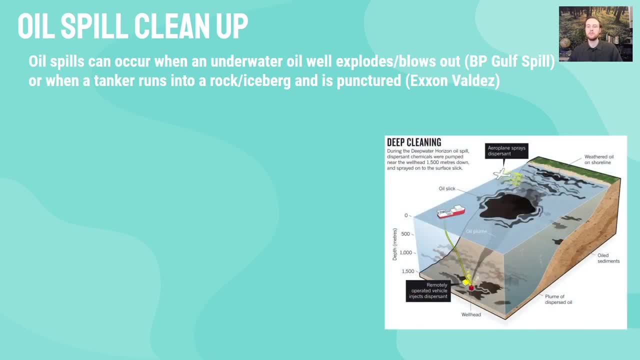 that oil can be spilled, And let's take a look here at how it can be cleaned up. Before we do that, though, I just want to point out in this diagram this is kind of an idea of how that Deepwater Horizon oil spill occurred. Basically, you can see, here at the ocean floor there's a 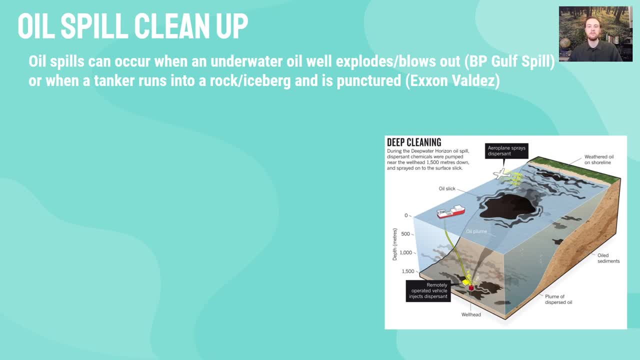 wellhead. there's an explosion in the wellhead and now we have what's called a plume- An oil plume is a really good example of an ape's vocab word That you should know. It's basically a column of oil migrating up through the water, and then it can. 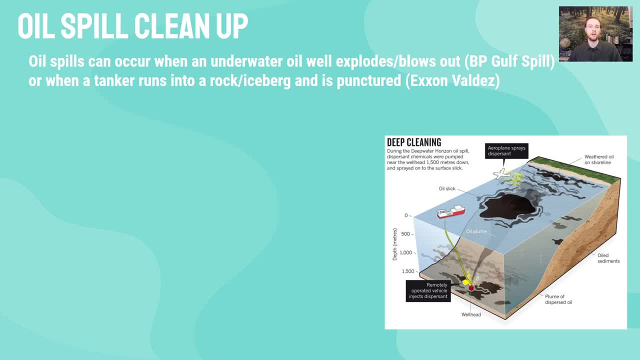 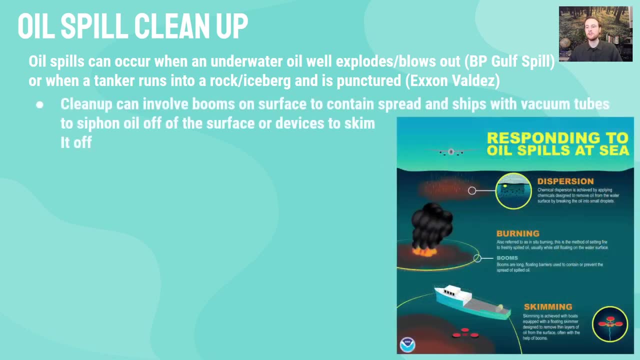 form an oil slick, which is a big patch of oil on the surface. So plume and slick- those are good ape's vocab words that you want to have down when it comes to oil spills. So the first thing that we can do is we can just try to use booms, which are these large plastic, almost like floating fences. 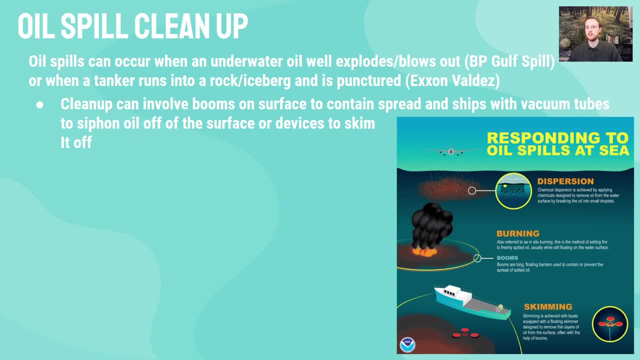 that can try to contain the oil. So we can see that on the bottom here where it says skimming. We're going to try to use a boom, a big plastic barrier, to contain the oil and then we can skim it off the surface or actually try to vacuum it off. So there's ships with pumps that could try. 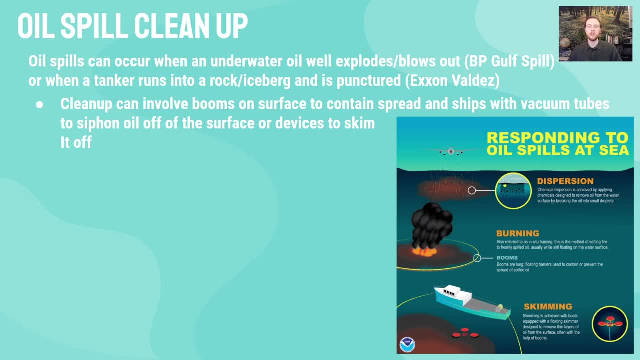 to suck the oil off the surface And that is probably the quickest way or the most you know immediate solution that people start to employ when there's an oil spill. We also have physical removal, So when it washes ashore it can just be physically removed from the rocks, from the sand. 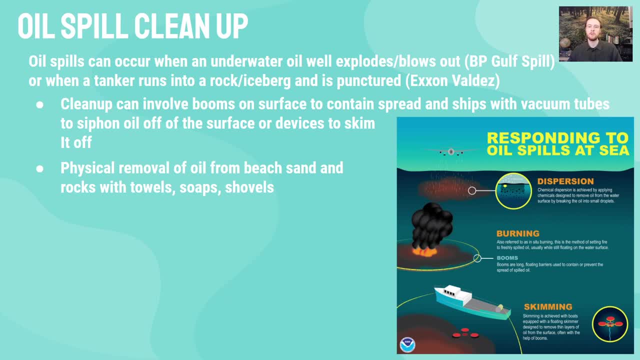 You can scoop it up, You can use detergent and towels to try to wipe it off rocks or clean it off birds or other organisms, And we also have chemical dispersants, And so these are going to be synthetic chemicals that humans make, and then we're going to spray them basically all over the oil spill. 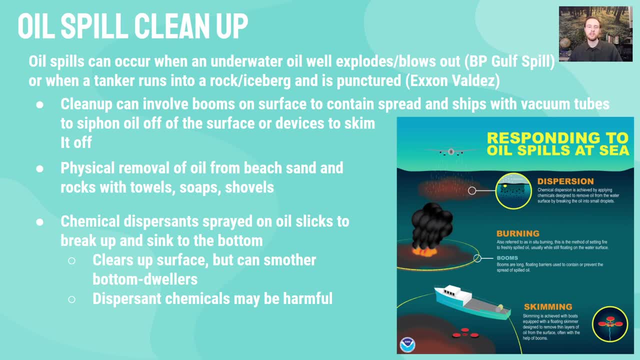 oftentimes of the plane, as you can see in this diagram, And the trick here is that they are just going to make the oil break up. They're almost like a soap or detergent, And so, like I said earlier and like I've said,